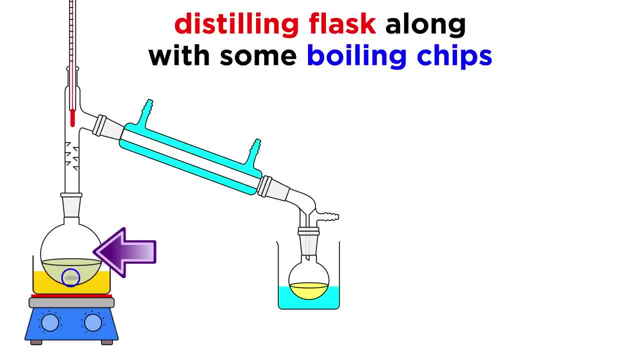 Our mixture will go in here along with a couple of boiling chips. This will sit above the heat source, be it a hot plate, Bunsen burner or whatever we are using. We bring the mixture to a gentle, boil and vapor is produced. 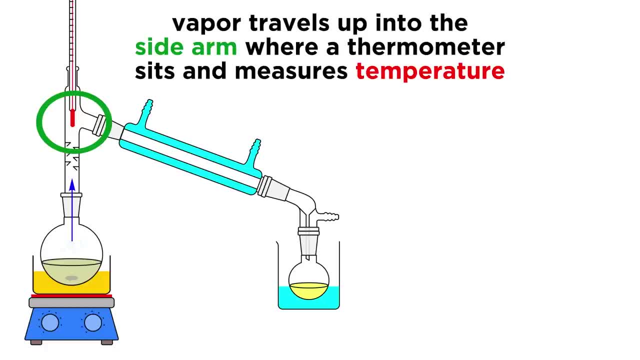 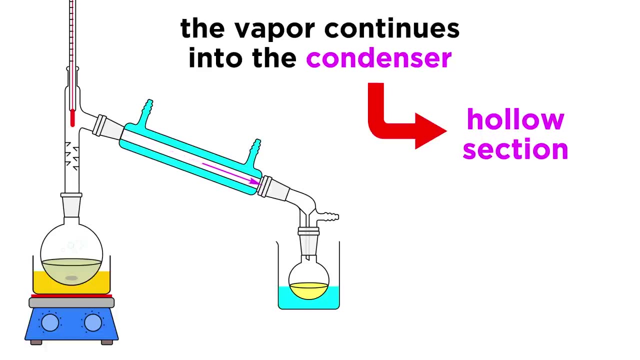 This vapor will rise into the side arm and a thermometer will sit here measuring the temperature of vapor. right as it approaches this horizontal section, The vapor continues into the condenser. This has a central hollow section where the vapor will pass, surrounded by another section. 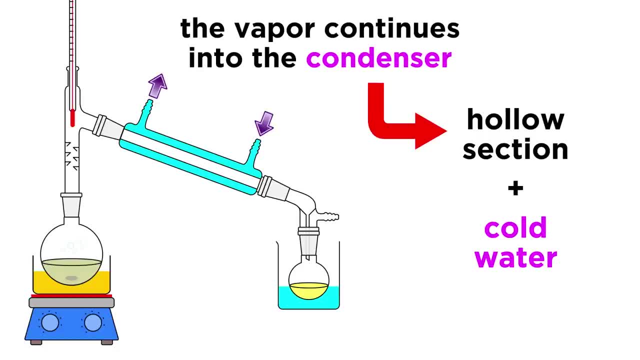 where cold water will enter on one side and then exit from the other. This will be constantly running and against the direction of the vapor. This cold water will cause the temperature inside the condenser to drop, so when the vapor enters this section it will condense back into a liquid. 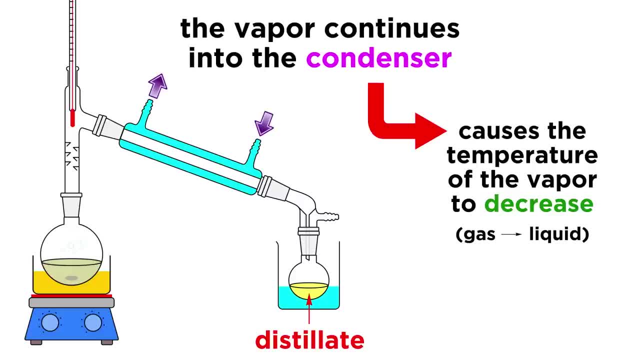 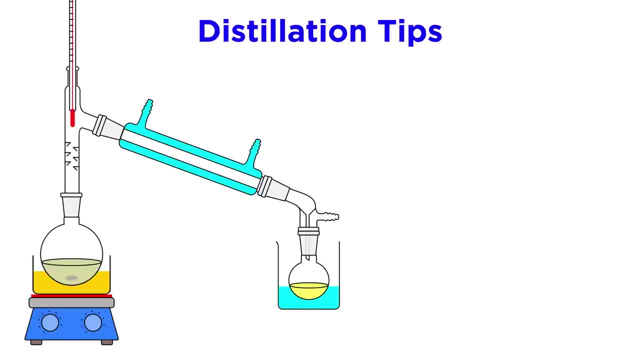 This liquid is called the distillate, And we will collect it in a receiving flask And just like that, separation is achieved. Now let's mention a few quick tips to make sure your distillation goes smoothly. First, make sure your distillation flask is not more than half full. 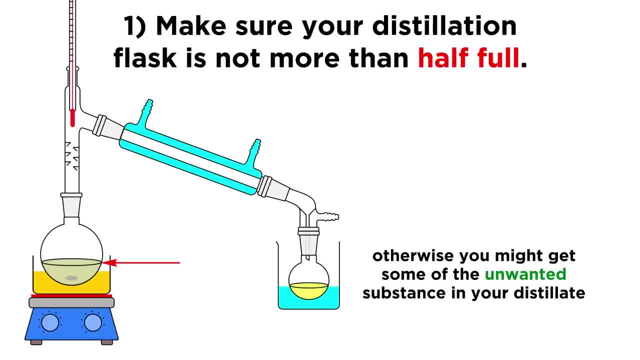 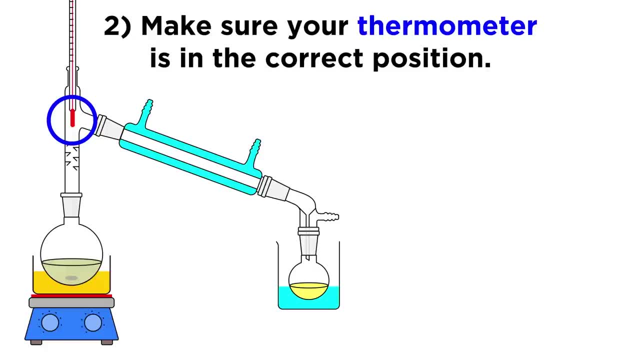 If it is too full, some of the unwanted substance might make it into the distillate. Second, make sure your thermometer is in the right position up here, as we want to measure the temperature of the vapor, not the water. This is important because if the temperature is too high, the vapor will not be able to. 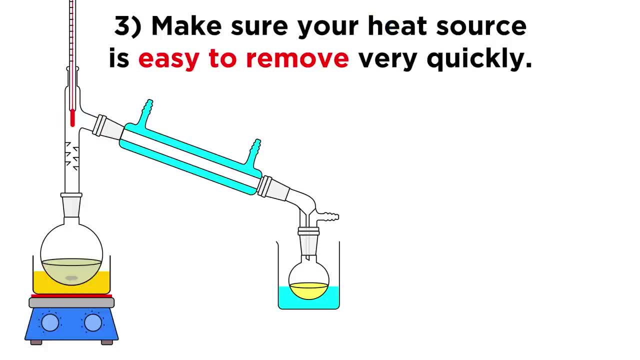 get into the liquid. Third, make sure your heat source is easy to remove very quickly. If it's a Bunsen burner, make sure the setup is such that you can just pull the burner away instantly. If a hot plate, make sure it's easy to loosen one clamp and pull things apart easily. 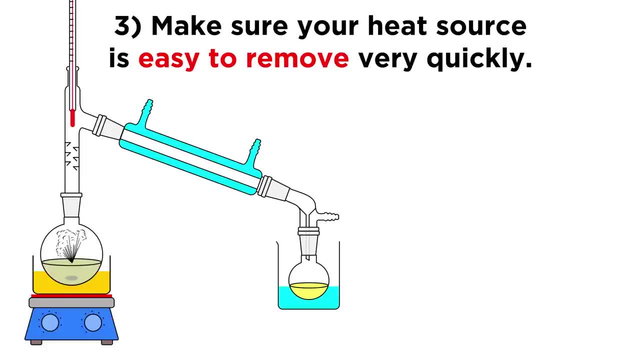 It's possible for the mixture to suddenly begin boiling violently and we need to remove the heat right away if that happens. Fourth, make sure every hot plate has a hot plate. Make sure every piece of glassware is clamped properly, especially the condenser. 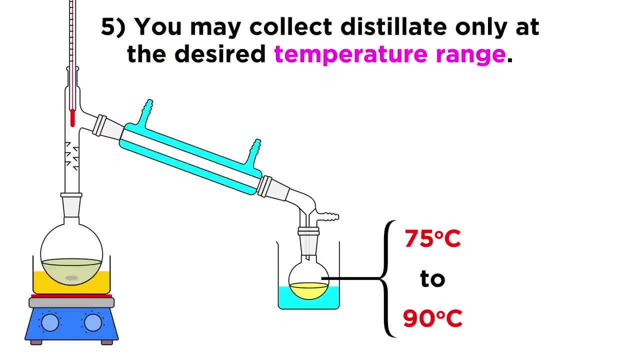 Clips should connect everything. And lastly, it's sometimes a good idea to just collect distillate at the desired temperature range that corresponds with the boiling point of what you want. This will minimize contamination. So we can see how this technique is useful for separations.